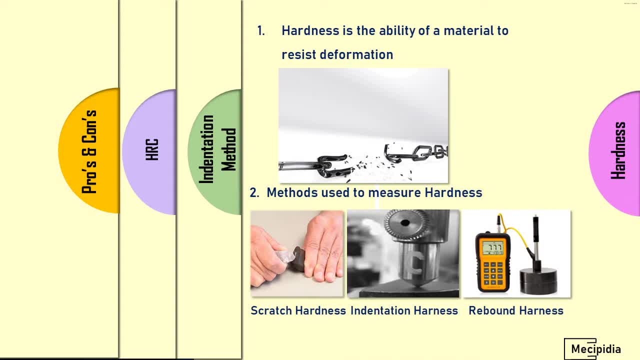 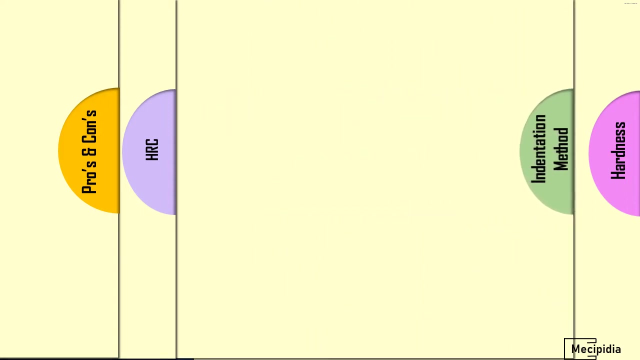 tip is applied with the force on the test piece. so the energy loss during elasticity, elastic deformation, it is measured as a rebound harness in automobile field majorly the indentation harness are being followed. so let us see that in detail. so test piece is intended until an impression. 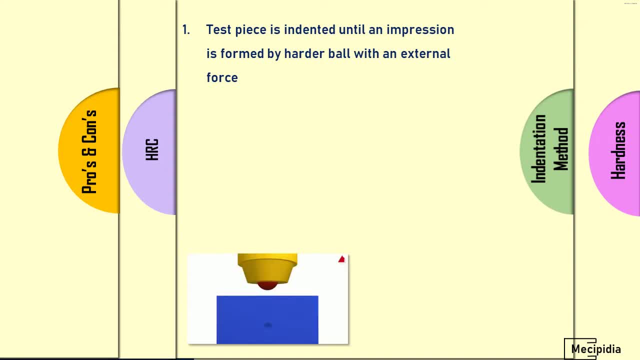 is formed by a harder ball with the external force. you can see the image below the ball with external force. it is applied on test piece so that creates the impression. that impression is called indentation. that indentation diameter is measured and evaluated in the indentation harness scale. so there are four our indentation harness. 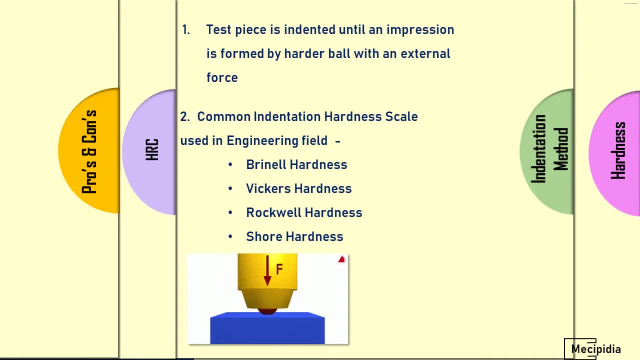 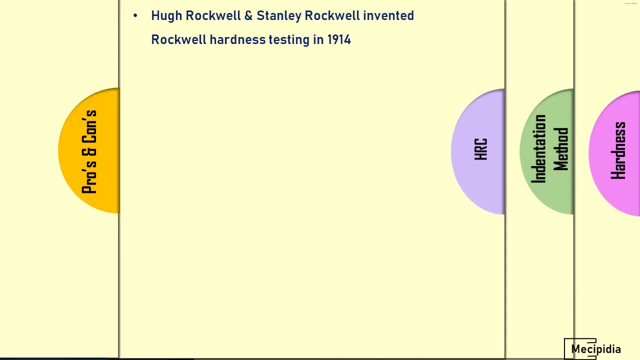 scale are being used in the engineering field. so first one is brinell harness and second Vickers harness, third Rockwell harness and final one is sore harness. so in this video we'll see about Rockwell harness in detail. Huck Rockwell and Stanley Rockwell invented the Rockwell harness testing in 1914. so it's basically. 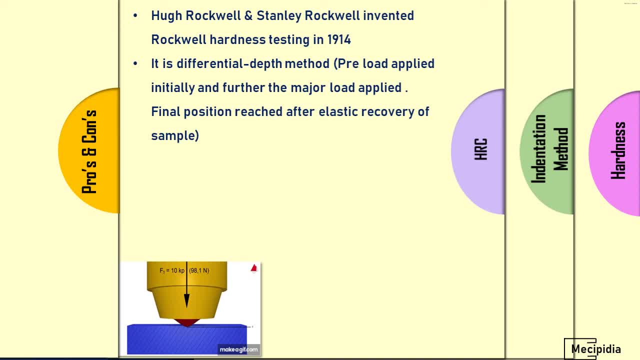 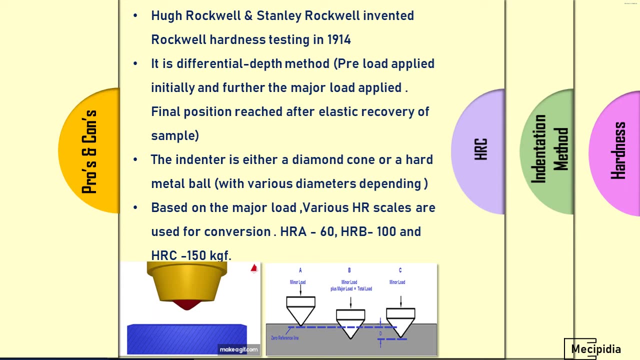 differential depth method, if you see the below image. so initially there is a preload is getting applied and further the major load is applied. so final position is reached after elastic recovery of sample, that that particular differential depth. it is measured only for the elastic recovery of sample. so the final position is, after elastic recovery of sample, the that particular differential. 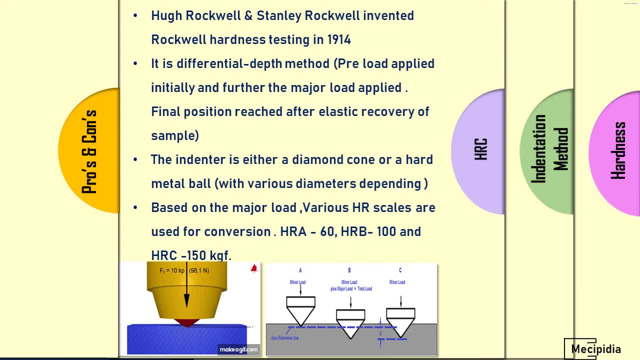 depth. it is measured only when the upper one is koried after Tubal approach. also today's example is is getting evaluated and it is just shown as a final hardness in the display, but in this case the intender is either diamond cone or hard barred metal based. 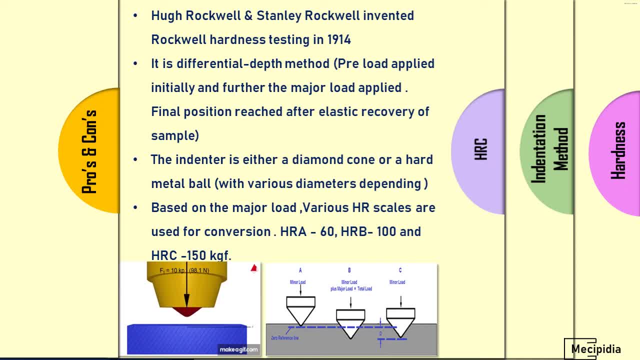 on the application and there are various scales are being used in Rockwell hardness and basically three scales are widely used: HRA, HRB, HRC. so that is based on the kg of load applied. so HRA is 60 kg load applied and HRB is 100 kg and HRC